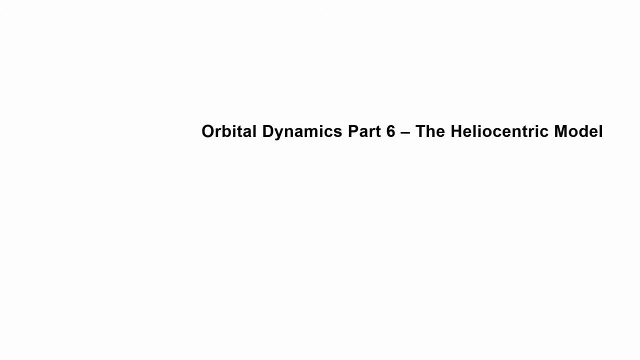 moon and earth believed the sun, because it was so large, had to be at the center of our solar system. His ideas didn't take hold. The idea was reintroduced by Copernicus and this time he introduced a more rational model. Even his idea was not embraced. 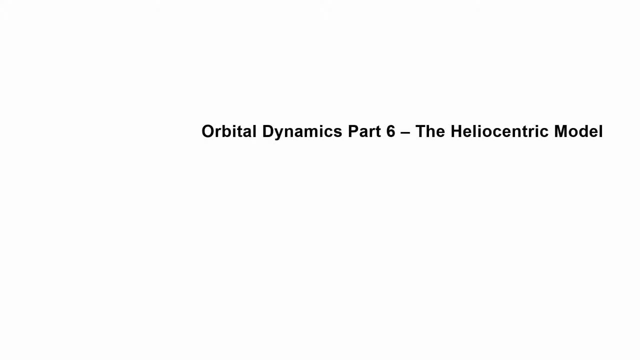 although he's credited with coming up with a heliocentric cosmological model. Why is this important to orbital dynamics? An earth-centric model is one way of looking at the solar system. In fact, we eventually have to convert other frames of reference to an. 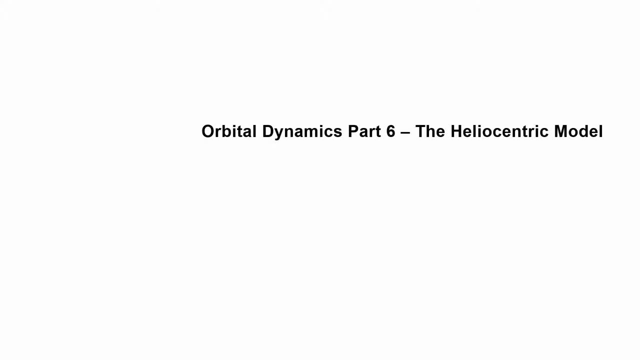 earth-centric frame, since earth is where we live. This means that an earth-centric model is not wrong per se. I'm going to show you that a solar-centric solar system- heliocentrism- is a better way to look at the solar system If the sun is not placed at the center of our 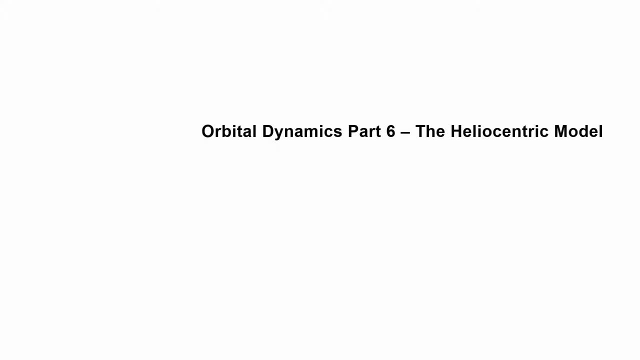 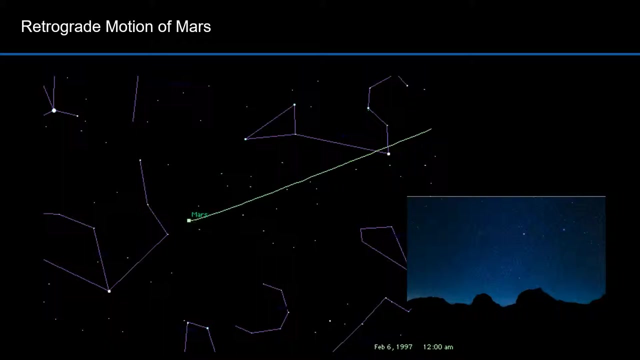 solar system, then it's hard to develop laws of physics- which I'll get into later- that back up the orbital motions that we observe. Later discoveries by Kepler and Newton could only have happened with a heliocentric model, As I mentioned in part one. ancient astronomers noticed that certain lights, as they called them, 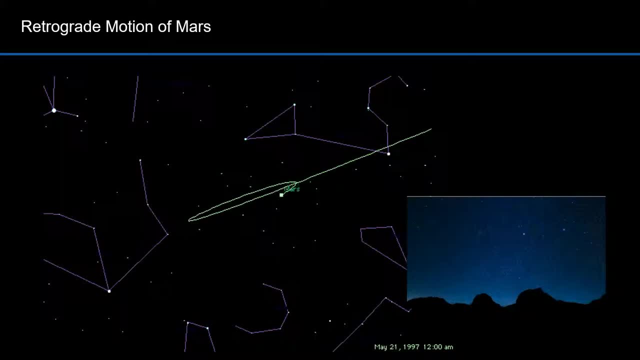 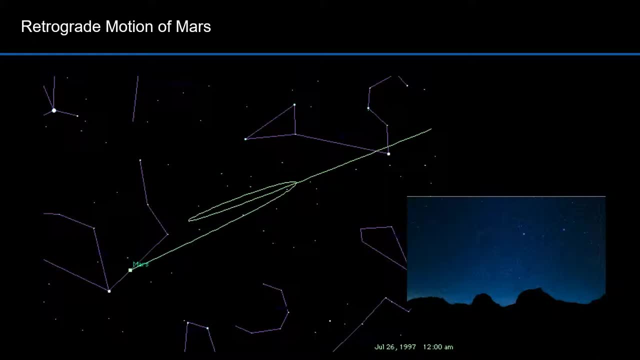 background. This animation is the path of Mars against the stellar background, from mid-October 1996 to late July 1997.. They called these lights Wanderers. In ancient Greek the word for Wanderer is planetes or planetes asterios. That's the root of our word planet. Notice that the path of Mars 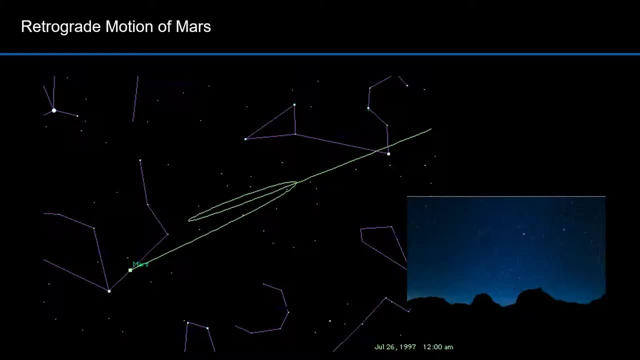 moves from east to west, changes direction and then changes direction again. Let's be clear: The stars and the planets generally move in the night sky from east to west. The stars and the planets generally move in the night sky from east to west. Mars goes along with this. 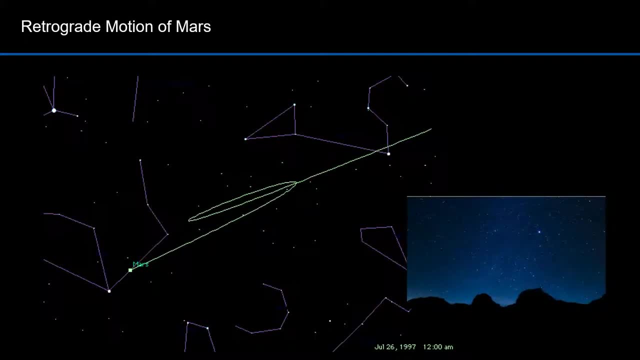 east-west motion. Every night, however, it creeps a bit to the west and then at some point it creeps eastward, and then it creeps westward again. The ancients wanted to understand this wandering motion. They also wanted to devise a system so they knew where to find the planets in the night sky on any 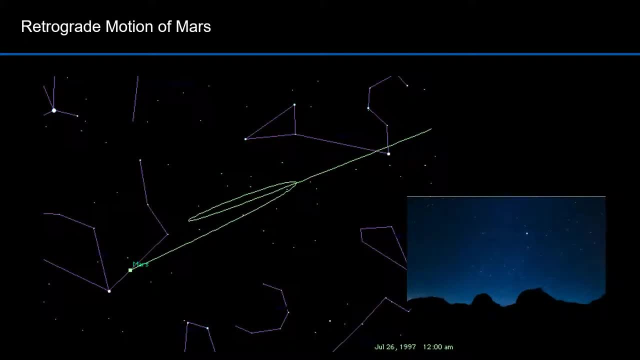 given night, Five planets were visible in this way: Mercury, Venus, Mars, Jupiter and Saturn. Uranus and Neptune weren't discovered until later. Pluto- much later. The ancients would have found them if they knew where they were. They're visible, but they're so far away they don't move much against the stellar background. 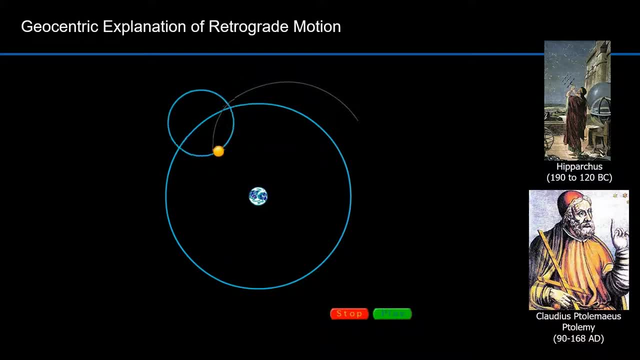 Ptolemy was a mathematician, astronomer, geographer, astrologer and poet. Hipparchus and later Ptolemy came up with a way to predict the motions of planets that accounted for their odd retrograde motion. The large circle is called the deferent, The smaller one is an epicycle. 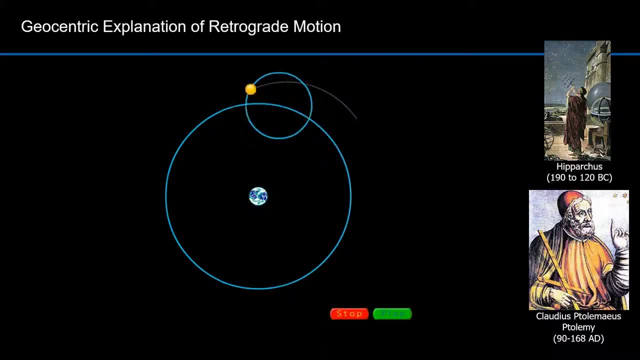 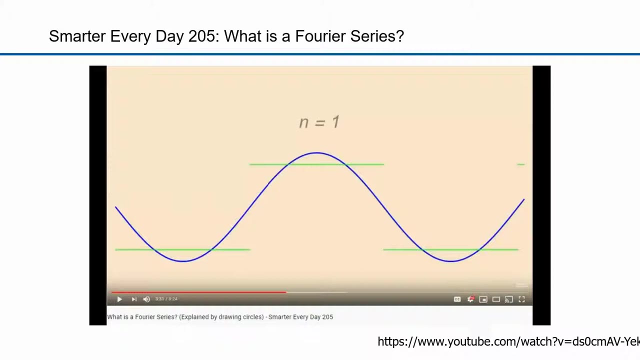 In this animation you can see how this model accounts for the observed retrograde motion of the planets. Importantly, this method enabled Ptolemy to derive very accurate tables of the planets, good enough for naked eye observations. Ptolemy's model is analogous to Fourier transforms. A Fourier transform decomposes a function of time. 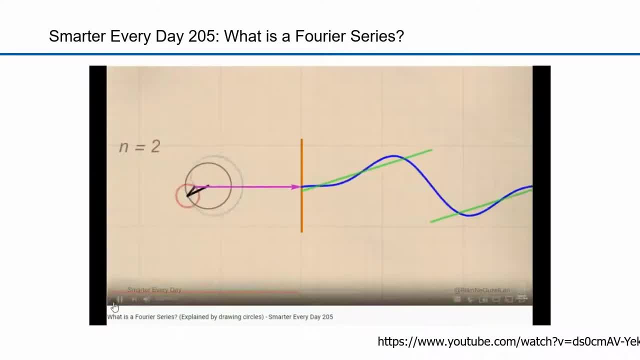 a signal into the frequencies that make it up, in a similar way to how a musical chord can be expressed as the frequencies or pitches of its constituent notes. There's a great video on YouTube that explains this. If you want to learn more about Ptolemy, you can click on the link in the description. 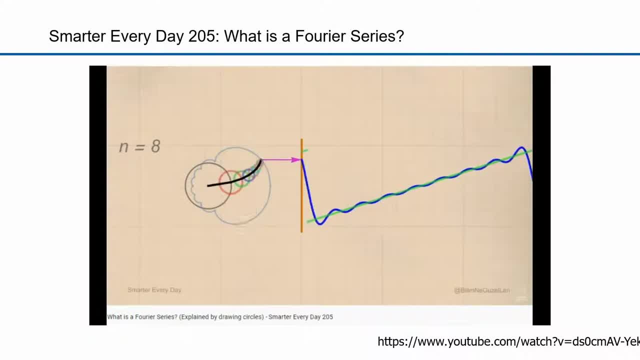 It's episode 205 of the Smarter Every Day series by Destin Wilson Sandlin. The video I'm showing here is an excerpt. What Destin teaches is that you can recreate almost any shape with a Fourier transform. In the animation I showed you, there was a 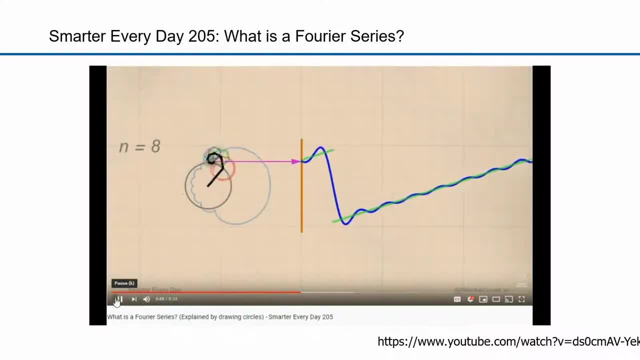 single deferent in one epicycle. Ptolemy also used a single deferent, but added multiple epicycles to increase the accuracy of his predictions. Each epicycle added more accuracy. That's essentially what you do with a Fourier transform: You keep. 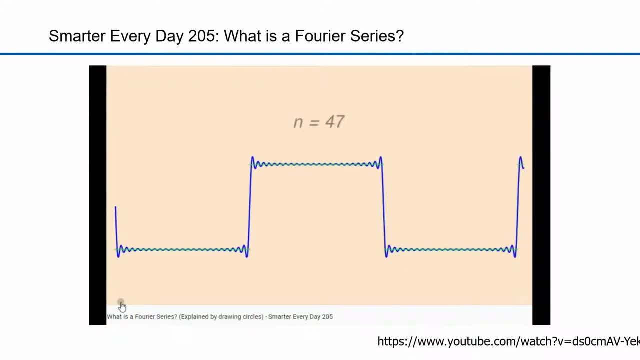 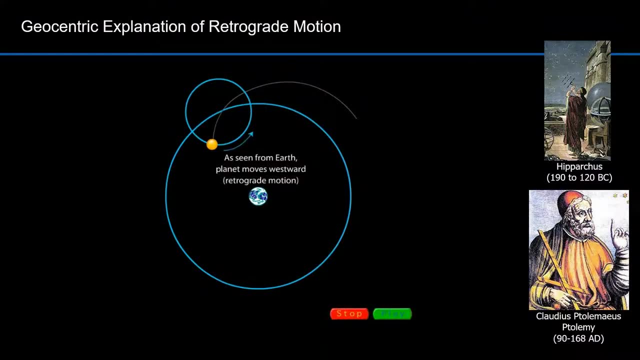 adding functions until the transform closely approximates the shape you're trying to recreate. Greek astronomers such as Hipparchus had produced geometric models for calculating celestial motions. Ptolemy developed astronomical models and convenient tables which could be used to compute the future or past position of the planets. 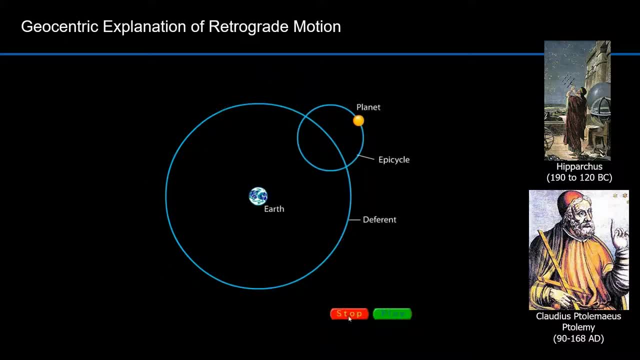 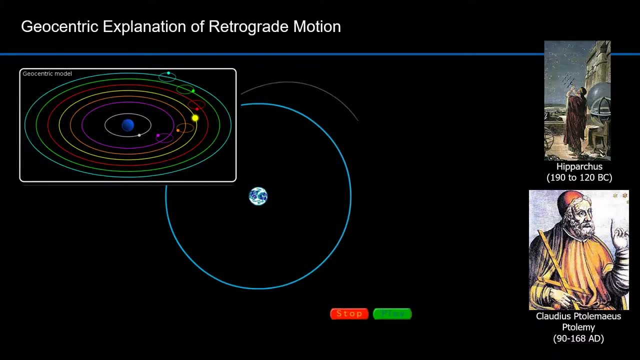 Ptolemy synthesized and extended Hipparchus's system of epicycles and circles to explain his geocentric theory of the solar system. Ptolemy believed the planets and sun orbited the earth in the following order: Mercury, Venus, Sun, Mars, Jupiter, Saturn. 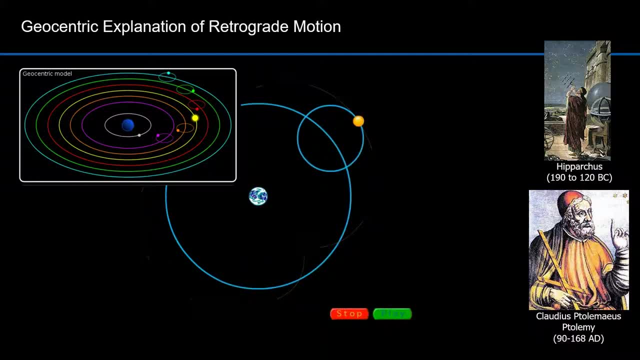 This system became known as the Ptolemaic system and predicted the positions of the planets accurately enough for naked eye observations. The Ptolemaic system made some ridiculous predictions about their motions, such as that the distance of the moon should vary by a factor of two. 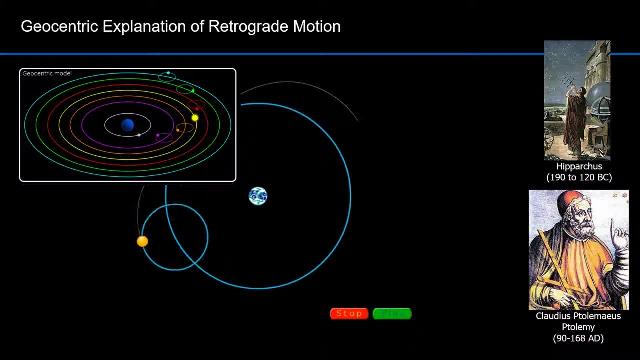 over its orbit, and you can see this erratic motion from this animation. While the Ptolemaic method predicted the locations of planets in the night sky very well, astronomers weren't able to devise laws of physics that explain the highly irregular motion. 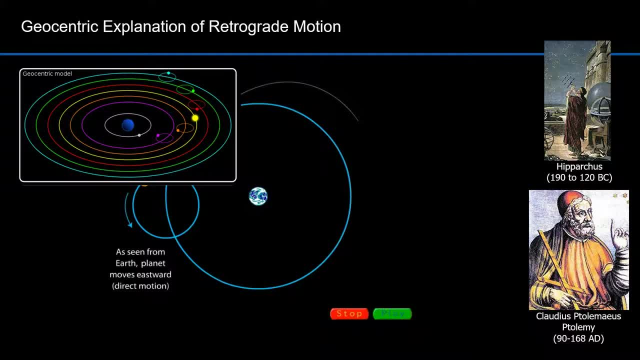 In fact, many believed this kind of irregular motion was not likely. These were mathematical models used to predict the locations of planets in the night sky, not a model of their motion. Orbital dynamics relies on an underlying physical model. This one didn't work and yet persisted for centuries. 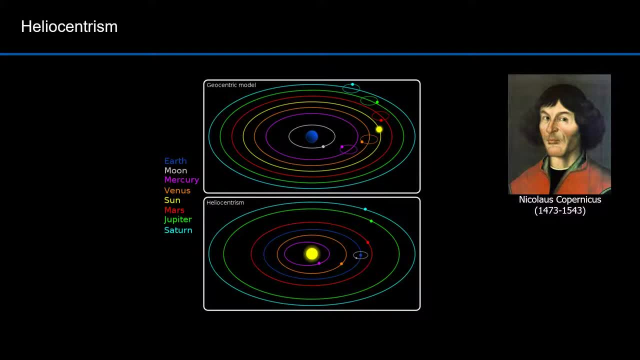 Nicholas Copernicus was a Renaissance astronomer and the first person to formulate a comprehensive heliocentric cosmology which displaced the earth from the center of the universe. Copernicus's epic book on the revolutions of the celestial spheres, published just before his death. 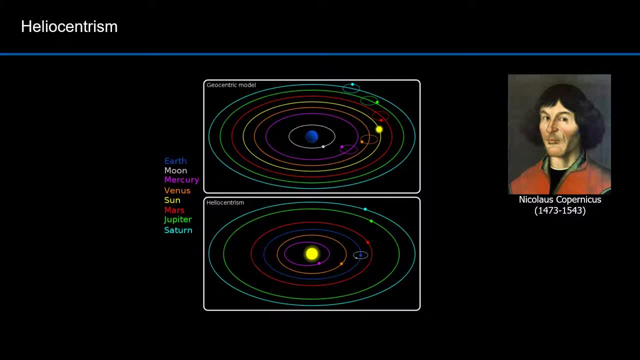 is often regarded as the starting point of modern astronomy. Copernicus Gra Ridge's theory of perturbation created an epiphany across the earth to him His heliocentric model with a look of the sun in the center of the universe. Coan and Pelvis may have explained celestial objects through the clear of the sun. 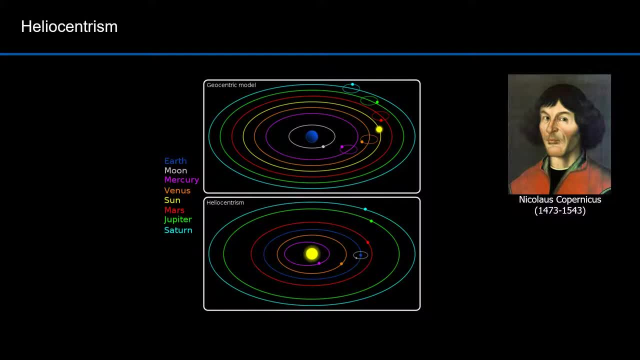 As Copernicus used to say in his book, all the spheres revolve around the sun as a midpoint, and therefore the sun is the center of the universe. What appears to us as motions of the sun arise not from its motion, but not from the motion of the earth. 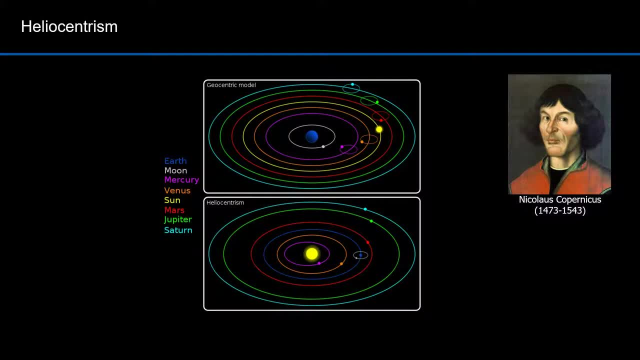 and its three myself sphere, which we revolve about: the sun. like any other planet, the earth has, then, more than one motion. the apparent, retrograde and direct motion of the planets arises not from their motion, but from the earth. the motion of the earth alone therefore suffices to explain so many apparent. 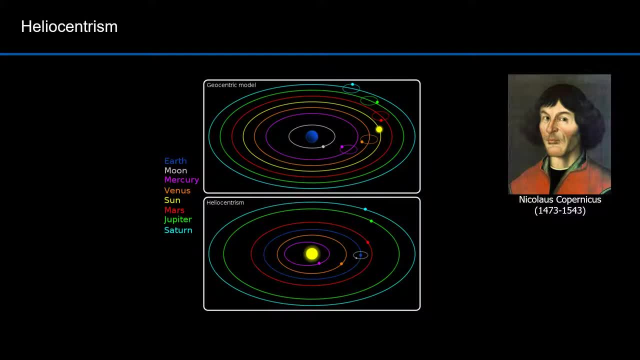 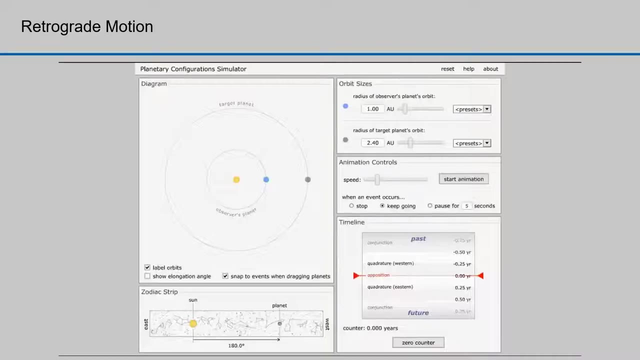 inequalities in the heavens. copernicus's theory was geometric and somewhat philosophical. he had no theory of physics to back it up. copernicus's theory enabled later discoveries, but the actual discoveries would have to wait for newton and galileo. copernicus explained the back and forth motion of the planets by putting the earth in an interior. 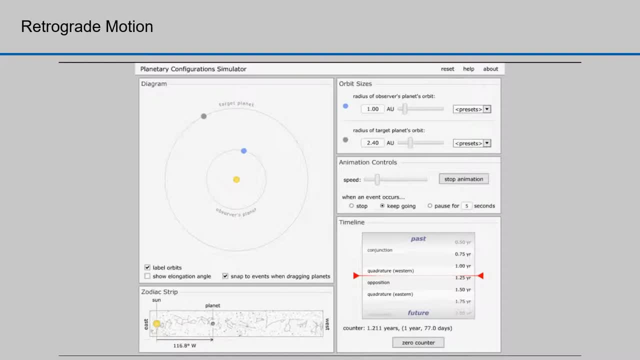 orbit and another planet in an outer orbit, like i'm showing this animation. if you look closely at the gray planet on the zodiac strip at the bottom of this animation, you can see the back and forth motion. if we make the earth an outer planet and the gray one an inner planet, like 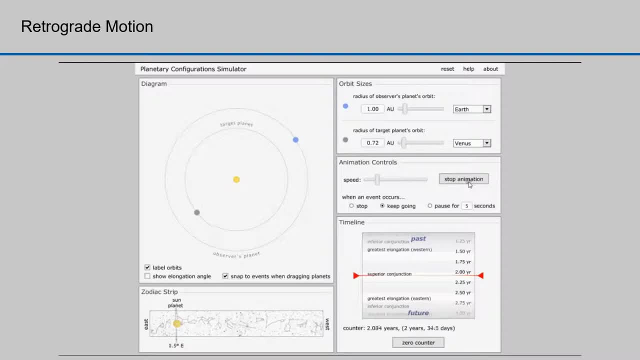 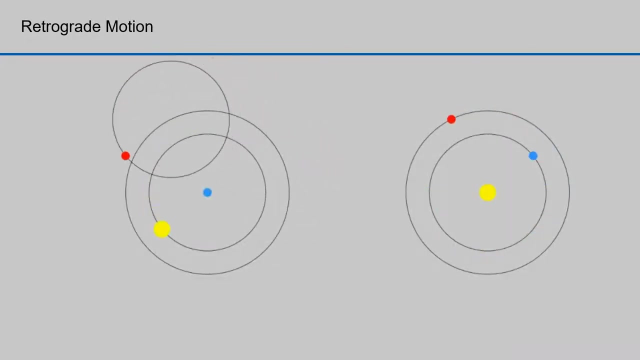 earth and venus. you'll see this back and forth motion as well. this is a much more intuitive explanation of the relative motions of the planets. the motions were now much simpler and much more intuitive. here's a comparison of the Ptolemaic and Copernican systems if we extend the line from the blue planet to the red. in each case you can. 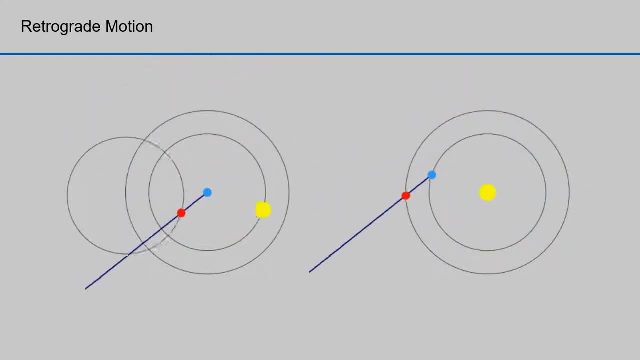 see, the two systems are the same and the two systems are remarkably similar. they don't predict the relative distance as well, but they do predict the relative direction of the red planet from the perspective of the blue planet. this is why the Ptolemaic system prevailed for so long. it was good at estimating locations of 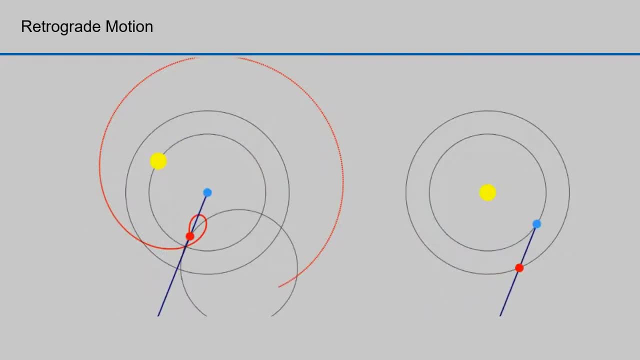 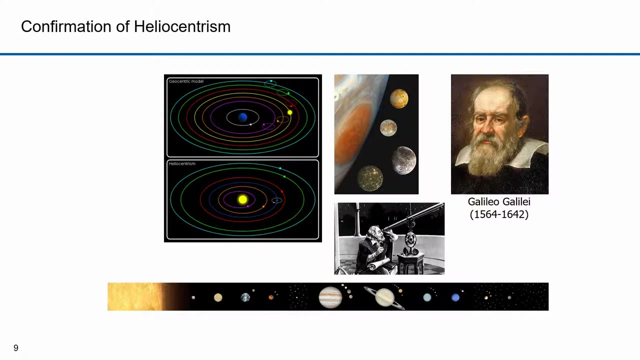 the planets relative to the earth. Galileo was an Italian physicist, mathematician, astronomer and philosopher who played a major role in the scientific revolution. his achievements include improvements to the in consequent astronomical observations and support for Copernicism. Galileo has been called the father of modern observational astronomy and the father of modern physics and the father of. 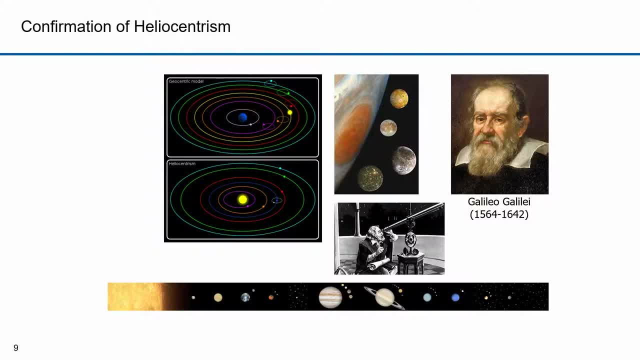 modern science. He built the first astronomical telescope, based on designs invented by Hans Lippershey in the Netherlands and improved to the point where it provided 30 times animation. On 7 January 1610, Galileo observed with his telescope what he described at the time. 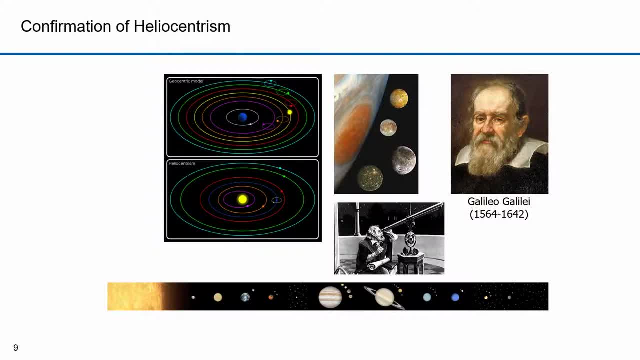 as three fixed stars, totally invisible by their smallness, all close to Jupiter and lying on a straight line through it. Observations on subsequent nights showed that the positions of these stars relative to Jupiter were changing in a way that would have been inexplicable if they'd really been fixed stars. On 10 January, Galileo noted that one of them had disappeared. 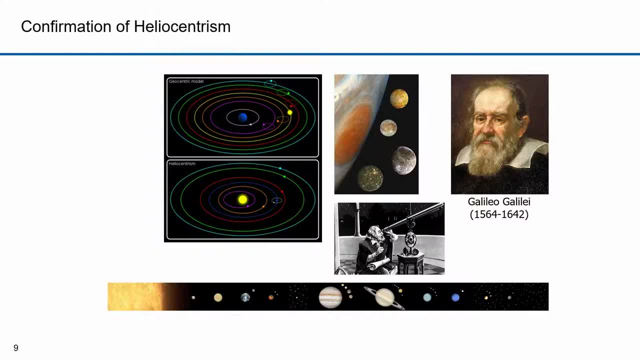 an observation which he attributed to its being hidden behind the stars. Within a few days, he concluded that these stars were orbiting Jupiter. He had discovered three of Jupiter's four largest satellites or moons. He discovered the fourth on 13 January. 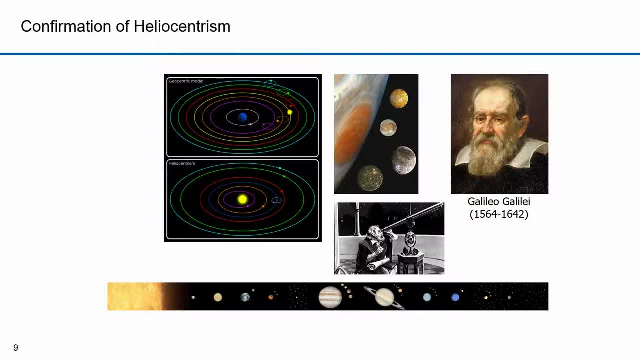 These satellites are now called Io, Europa, Ganymede and Callisto, later renamed to the Galilean satellites in his honor. His observations of the satellites of Jupiter created a revolution in astronomy. A planet with smaller planets orbiting it did not conform to the principles. of a reciprocal universe. This is why Galileo's observations of the satellites of Jupiter created a revolution in astronomy: A planet with smaller planets orbiting it did not conform to the principles of a reciprocal universe. This is why Galileo's observations of the satellites of Jupiter created a revolution in astronomy: A planet with smaller planets orbiting. it did not conform to the principles. 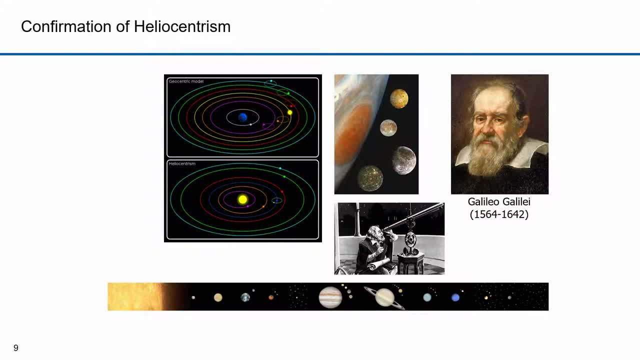 of a reciprocal universe. This is why Galileo's observations of the satellites of Jupiter created a revolution in astronomy, which held that all heavenly bodies should circle the earth. many astronomers and philosophers initially refused to believe that Galileo could have discovered such a thing. Galileo also observed Venus as it went through its phases. 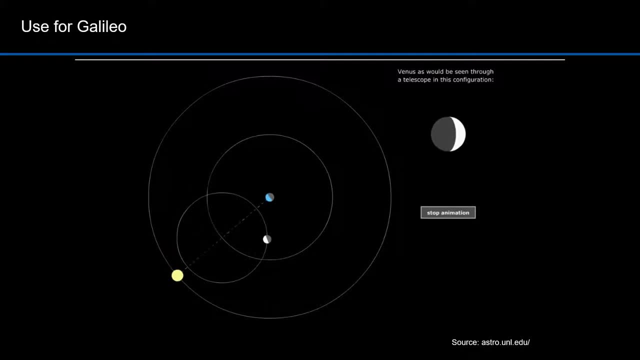 Here's Venus and the sun orbiting the earth in a Ptolemaic system. Notice that you never see a full Venus. That isn't possible in this system. Notice too that when that, when Venus is new, it's either very large or very small. It's at its largest when it's closest. 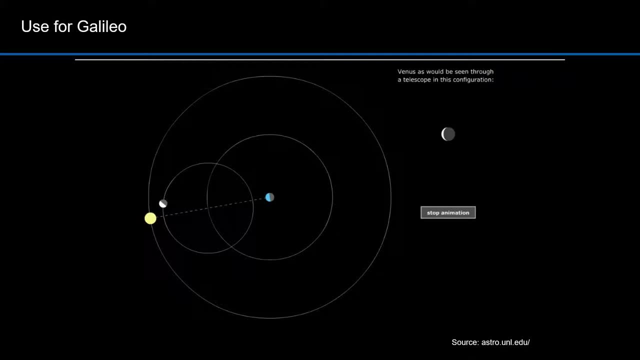 to the Earth, and at its smallest, when it's farthest from the Earth and closest to the Sun. In both cases, it's a new Venus, similar to a new Moon that's totally dark. This is what the Ptolemaic system predicted. 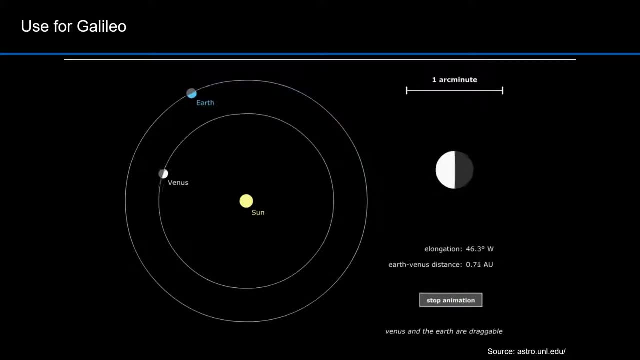 Here's what Galileo actually observed Over the 224-day orbital period of Venus. Galileo observed it going through all phases, including full illumination. The Ptolemaic model didn't allow for that. The Copernican model did Also notice that it's at its biggest. 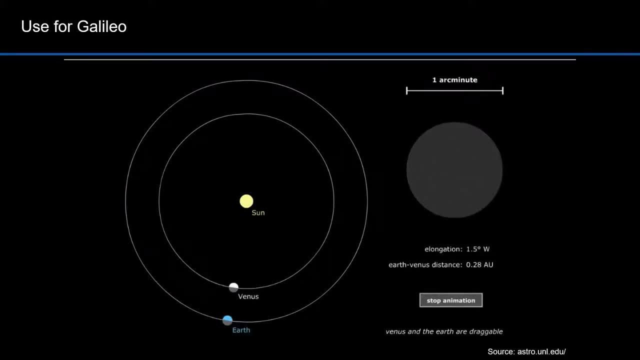 up to an arc minute as it becomes new and then shrinks when it becomes full. This could only happen if Venus and Earth orbited the Sun. with Venus in an interior orbit, You could construct a Ptolemaic model that allowed for these phases. 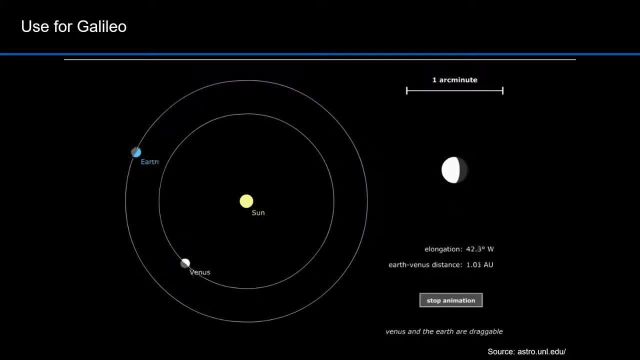 but it wouldn't predict the location of Venus with any accuracy. If you went with a model that predicted the locations of Venus, it didn't account for the phases. This is the Ptolemaic model. This discovery, along with Moon's orbiting Jupiter. 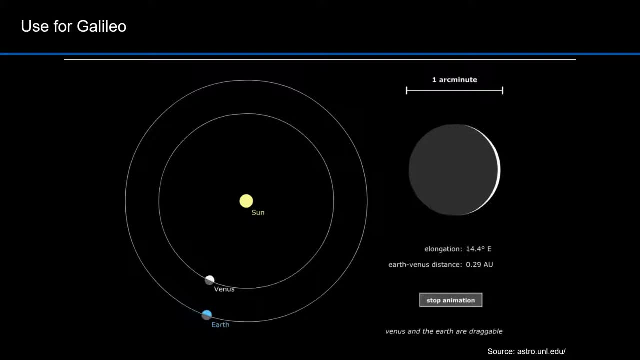 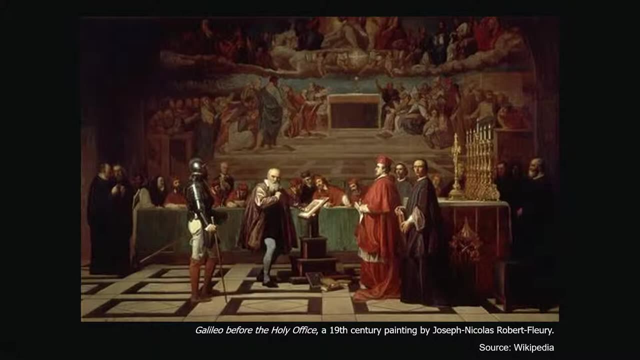 led Galileo to believe that the Sun had to be at the center of the Solar System. This is an edited excerpt from Wikipedia. Galileo's championing of heliocentrism was controversial when most subscribed to either geocentrism or the Ticonic system He met with. 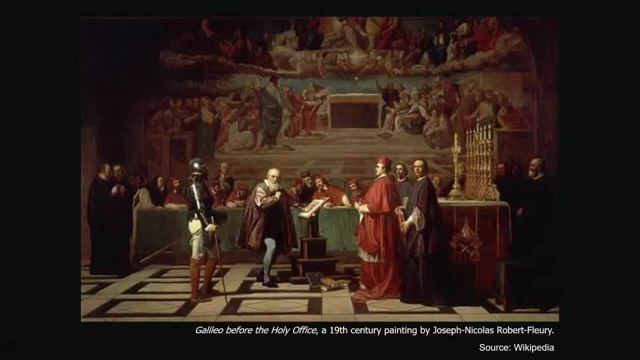 opposition from astronomers who doubted heliocentrism due to the absence of an observed stellar parallax. The matter was investigated by the Roman Inquisition in 1615, which concluded that heliocentrism was false and contrary to Scripture, placing works advocating the 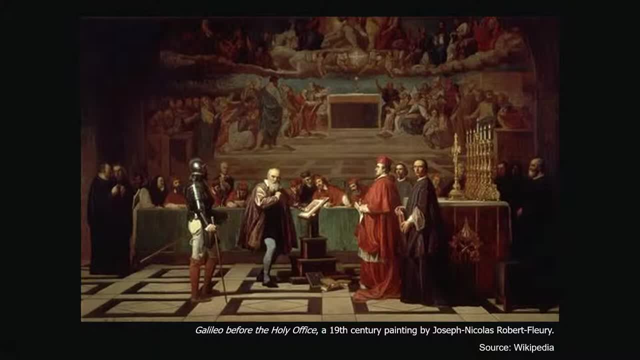 Copernican system on the Index of Banned Books and forbidding Galileo from advocating heliocentrism. Galileo later defended his views in dialogue concerning the two chief world systems, which appeared to attack both Pope Urban VIII, alienating the Pope, and the Jesuits, who had both. 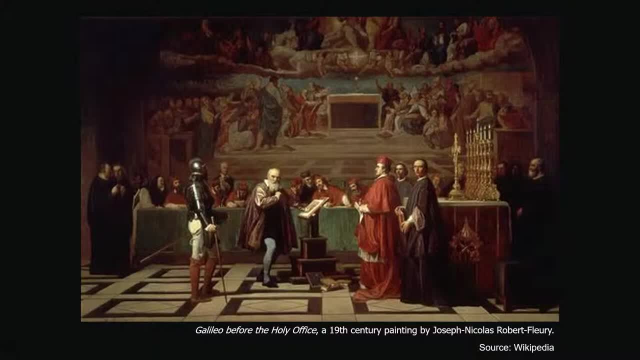 supported him up until that point. He was tried by the Holy Office and found vehemently suspect of heresy. He was forced to recant and spent the rest of his life under house arrest. According to popular legend, after recounting his theory, Galileo allegedly muttered the rebellious. 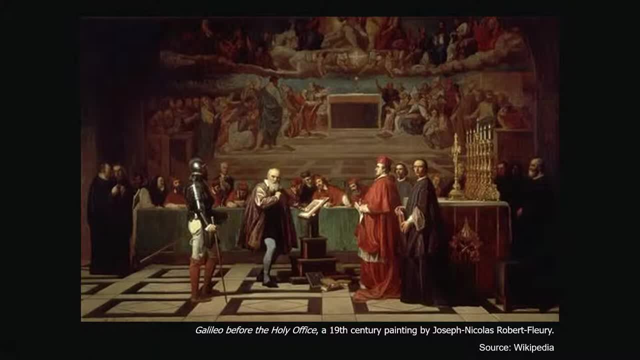 phrase and yet it moved. But the only evidence that he ever said that comes from a 1640 painting in which the words were hidden until restoration work in 1911.. The first written account dates to a century after his death, so he probably didn't say it. 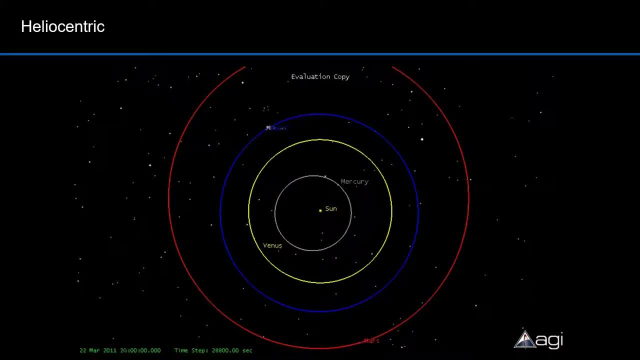 Here's what an actual heliocentric model looks like. These are the interior planets: Mercury, Venus, Earth and Mars. This is the model we're used to and have pretty much accepted. This is the Copernican model that Aristarchus first suggested. 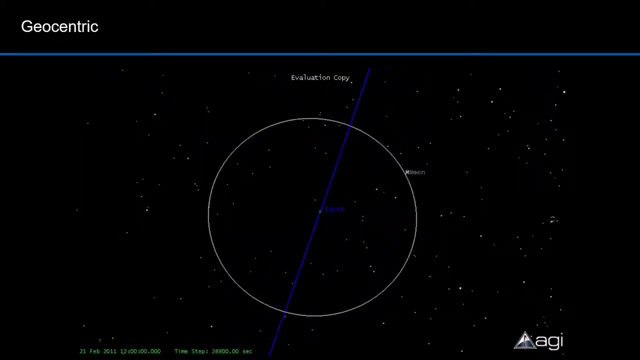 Here's a real geocentric model that predicts the locations of the sun and planets accurately. I put the Earth at the center of the solar system and have the sun and planets orbiting it. The Ptolemaic model works that the planets are on a single deferent that's in line with the sun's. 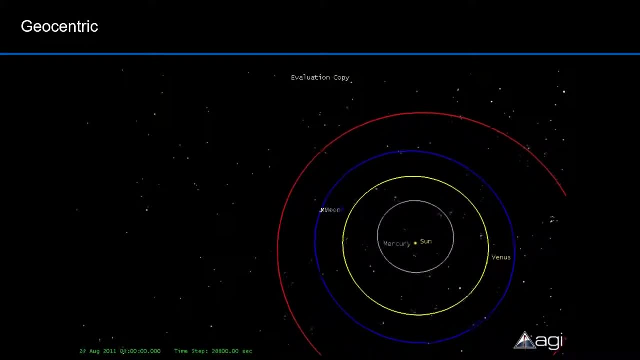 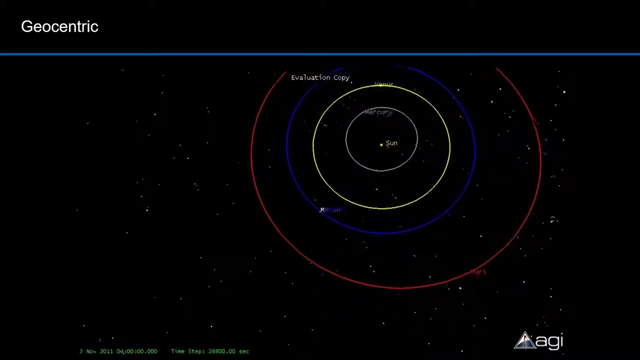 path around the Earth. Each planet then gets its own epicycle. Thank God Ptolemy didn't come up with this model. It would have been very accurate but not very intuitive. It's not that this geocentric model is wrong and the other heliocentric model is right. Both are valid. 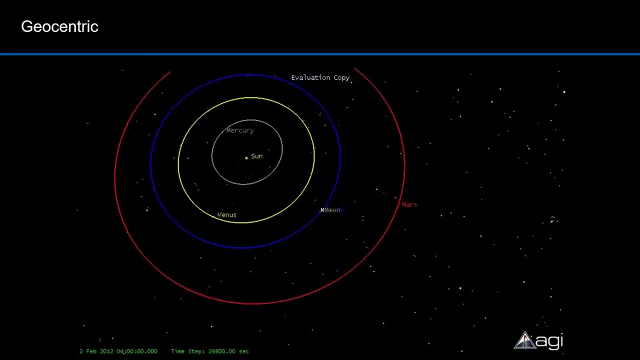 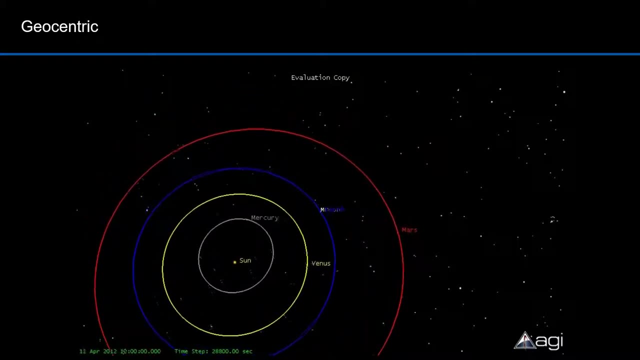 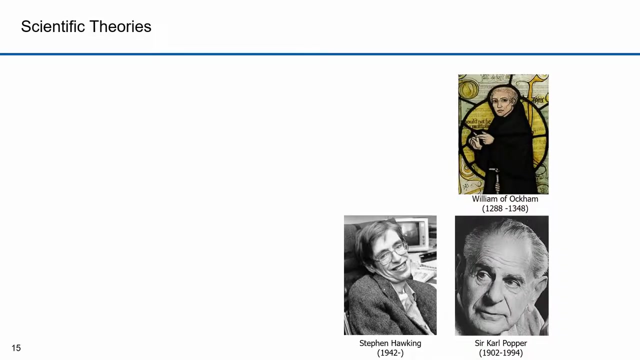 models for predicting the locations of planets in the solar system. The heliocentric one is more intuitive and opens up more advanced theories of physics. It's a preferred model, not necessarily the right model. Stephen Hawking in A Brief History of Time states: 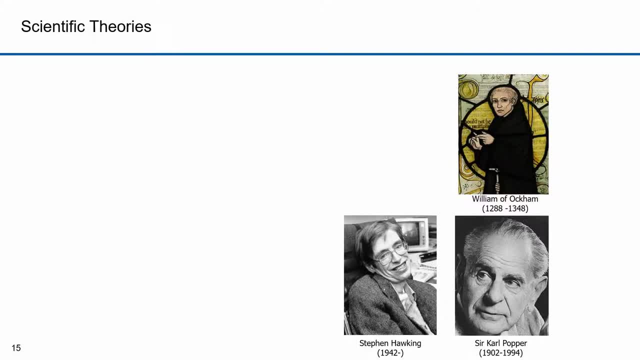 a theory is a good theory if it satisfies two requirements: It must accurately describe a large class of observations on the basis of a model that contains only a few arbitrary elements, and it must make definite predictions about the results of future observations. He goes on to state: any physical theory is always provisional, in the sense that 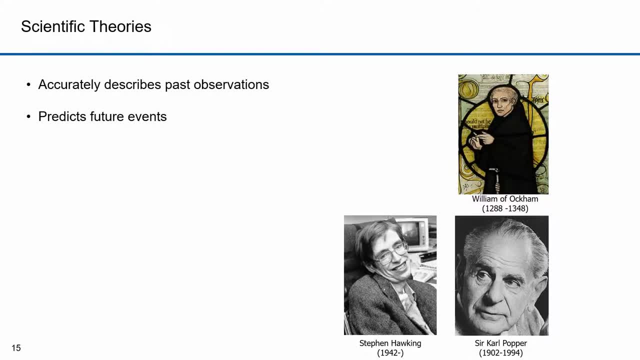 it's only hypothesis. You can never prove it. No matter how many times the results of experiments agree with some theory, you can never be sure that the next time the result will not contradict the theory. On the other hand, you can disprove a theory by finding: 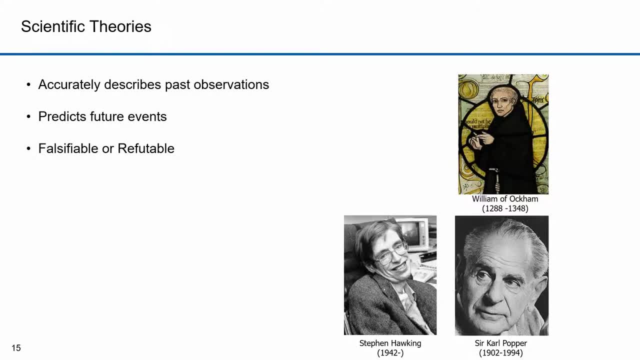 even a single observation that disagrees with them. The unprovable but falsifiable nature of theories is a necessary consequence of using inductive logic. The Scientific Philosophy didn't originate with Stephen Hawking. It was developed by Sir Karl Popper. He coined the term Critical Rationalism to describe his 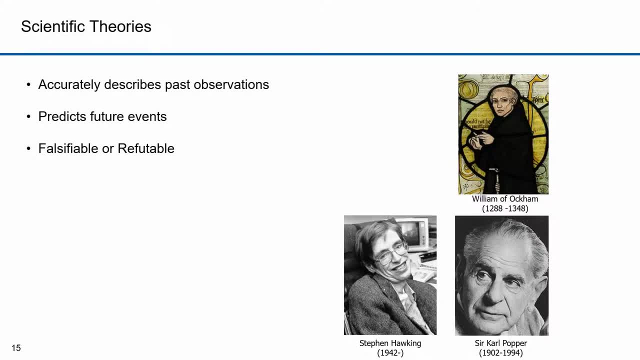 philosophy. Popper held that scientific theories are abstract in nature and can only be tested in directly by reference to their implications. Scientific theory, and human knowledge generally, is irreducibly conjectural or hypothetical and is generated by the creative imagination in order to solve problems like how to determine. 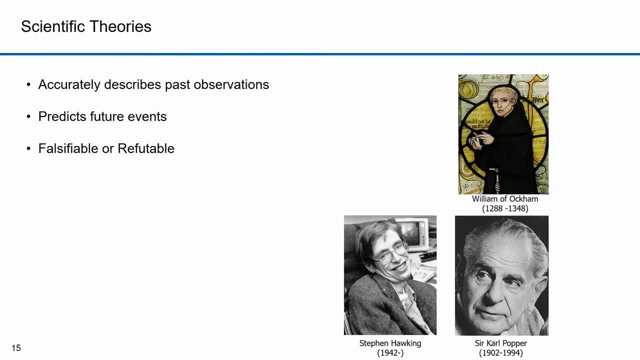 the future positions of planets. No number of positive outcomes of experimental testing can confirm a scientific theory explicitly. A single counterexample can refute a theory, however. it shows the theory from which the implication is derived to be false. A theory being falsifiable does not mean it has been proven false. rather, it means that 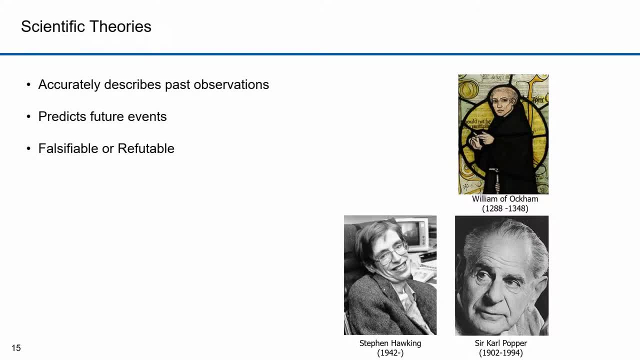 it can be shown by observation or experiment to be false. Some use the term refutable, others use the term testable. Popper's asymmetry between verification and falsifiability lies at the heart of his philosophy of science. It inspired him to take falsifiability as his criterion of demarcation between what 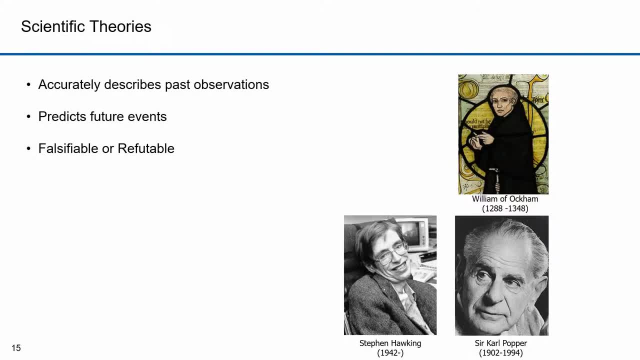 is and is not genuinely science. A theory should be considered scientific if, and only if, it is falsifiable, refutable or testable. Asserting a belief that cannot be tested is thus not a scientific theory. The fourth criterion for scientific theories embraces a concept called Occam's Razor. 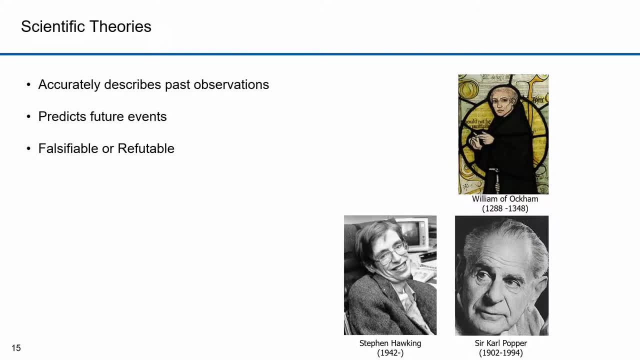 It's a term coined by philosophers that came after Sir William of Ockham. that refers to distinguishing between two hypotheses, either by shaving away unnecessary assumptions or cutting apart too similar. So what is scientific theory? The atomic amount of the earth on the planet Builder has been classified as not a scientific 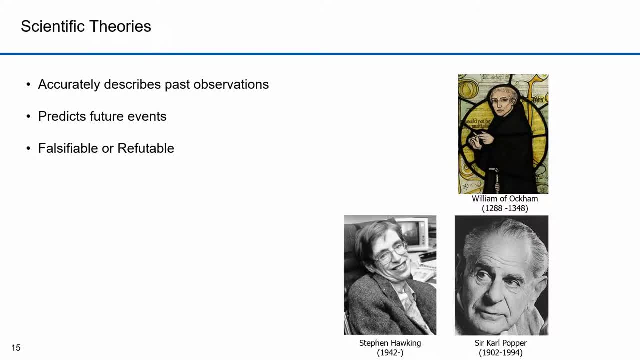 theory. In fact, it has been classified as a study of Earth's exact size. What does scientific theory imply? The theory that a single person can form a star, with its entire surface being an elliptic system in one individual, can be used to calculate the mass of the solar system. and 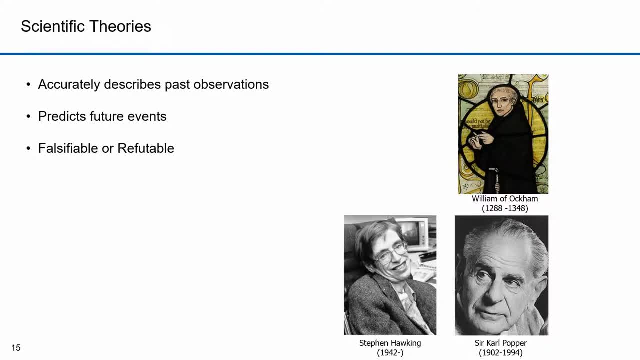 an Earth system than the heliocentric system. If you compare the math required for the Copernican system versus that required for the Ptolemaic system, Copernicus is far simpler. It's not that geocentrism is wrong. 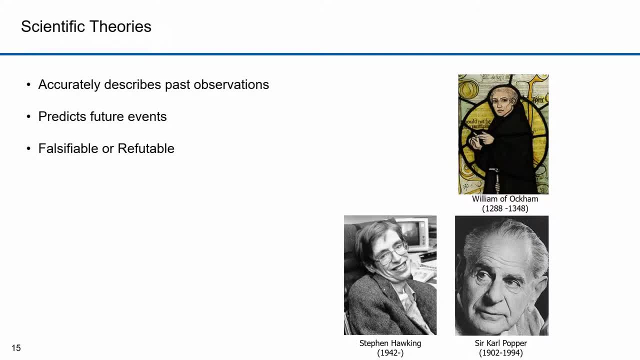 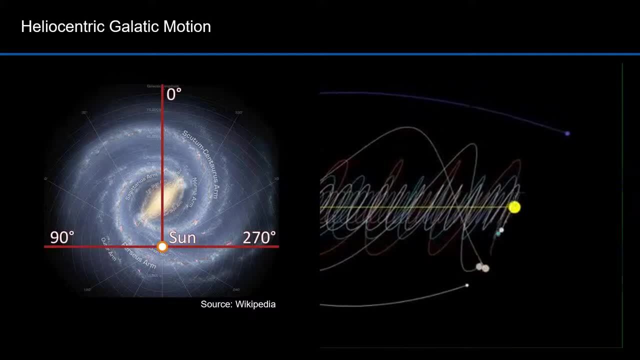 Geocentrism is simpler, more intuitive, and that's why it's preferred. Strictly speaking, the solar system is not static. It's orbiting the center of the galaxy. This video depicts the motion of the solar system through the galaxy.